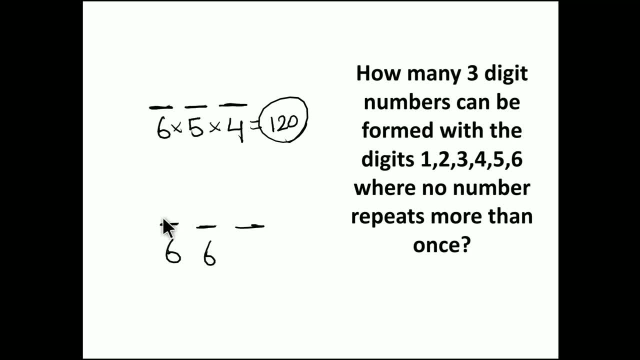 Second place can also be filled in 6 ways, Because if I fill the first place with 5, I can also fill the second place with 5.. Third place can also be filled with 5.. So we can simply say it is 6 x, 6 x 6.. 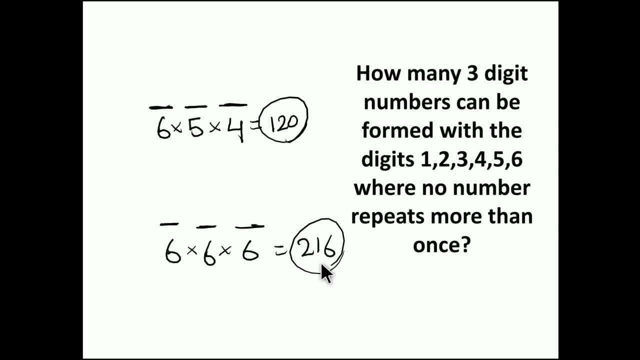 So 6 x 6 x 6 is nothing but 216.. So 216 3 digit numbers can be formed with the digits 1 to 3, where repetition allowed. But for this question 120 is our answer. So 120 3 digit numbers can be formed without repetition from the digits 1 to 6.. 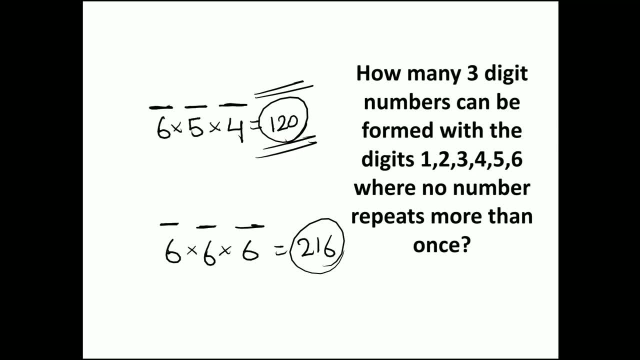 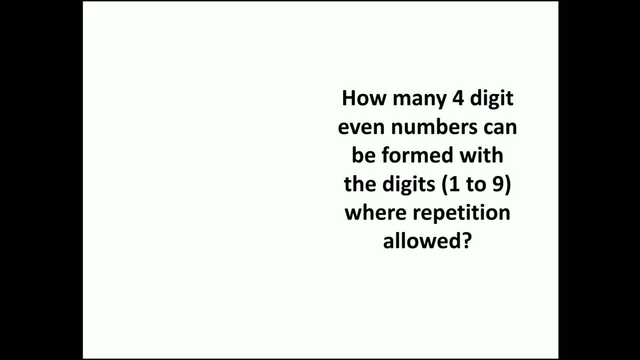 Hope you understood the concept right. Moving to second question of the video, How many 4 digit even numbers can be formed with the digits 1 to 9? where repetition allowed From 1 to 9, we totally have 9 numbers. 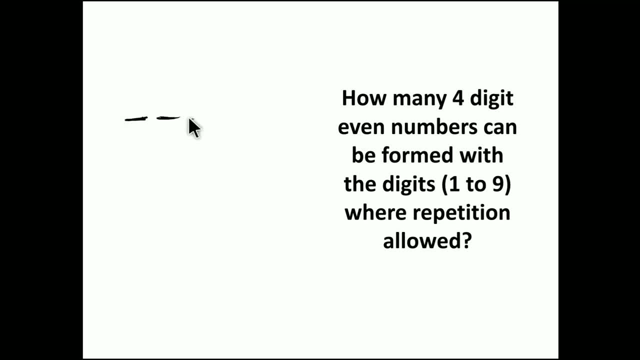 From this we have to frame 4 digit even number For even number. the condition is: last digit should be obviously an even number From 1 to 9, we have the even numbers 2,, 4,, 6, 8.. 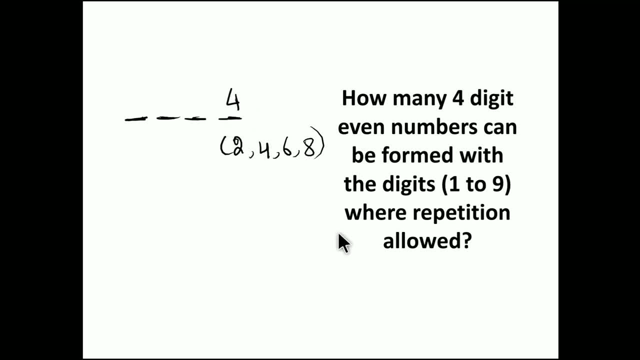 So last place can be filled in 4 ways And in question it is given repetition allowed. So repetition allowed in the sense the same number can be repeated for any number of time. So first place can be filled by any one of these 9 digits in 9 ways. 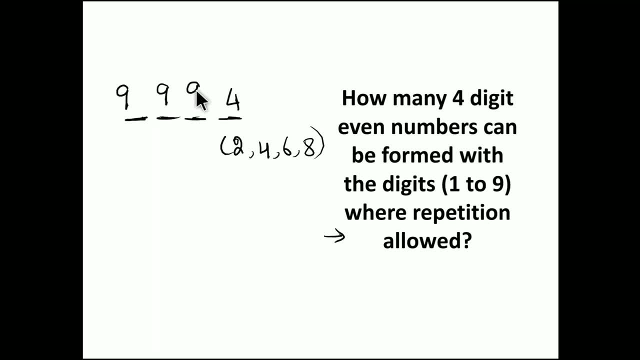 And second place can also be filled in 9 ways. Third place can also be filled in 9 ways, But fourth place should be filled in only 4 ways, because we have only 4 even numbers here. So 9 x 9 x 9 x 4 is our answer. 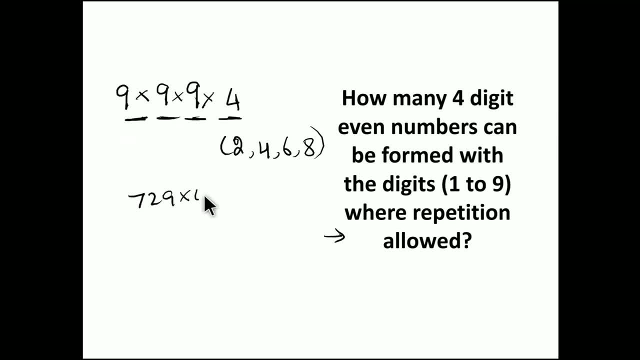 So 9 cube is 729.. 729 x 4 is our answer. So 6 x 3 is 8.. 1 is 829.. So here we totally have 9.. So here we totally get 2916, 4 digit, even numbers from the digits 1 to 9, where repetition allowed. 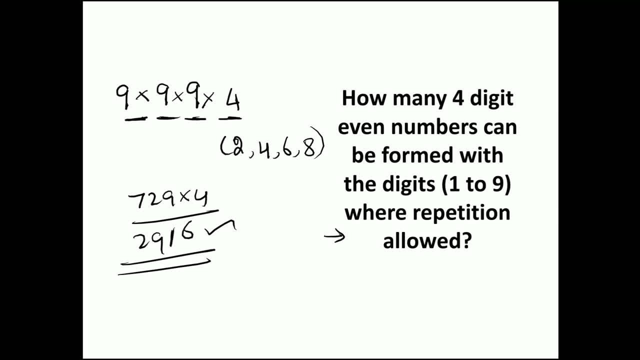 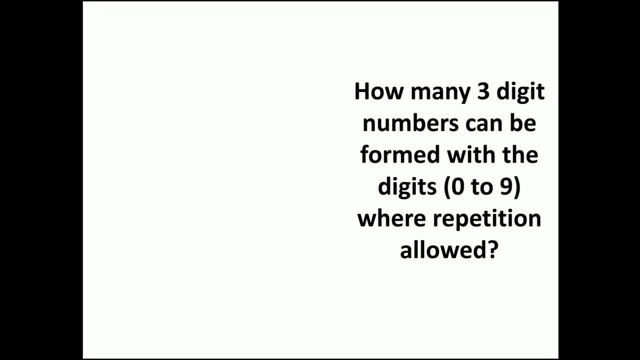 Hope you understood the concept right. Moving to third question of the video: How many 3 digit numbers can be formed with the digits 0 to 9? where repetition allowed 0 to 9, we totally have 10 digits right. 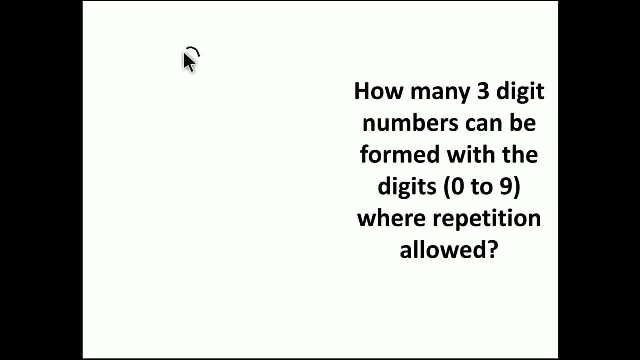 Before solving this question, you have to understand the concept 980.. For example, if you take 980.. It's a 3 digit number. right Now, if you have a number 089.. Is it a 3 digit number? 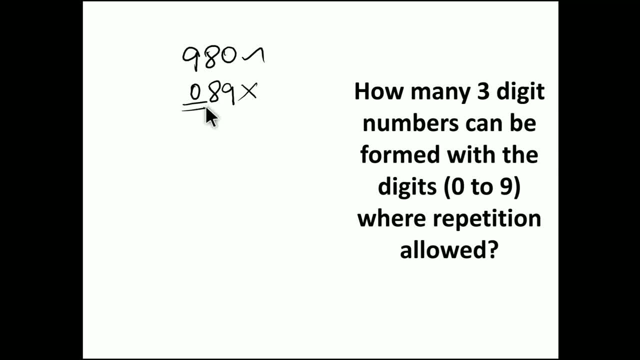 No, obviously not. It's a 2 digit number because in first place you have 0. So first place cannot be filled by 0. So if you fill the first place with 0, it will become a 2 digit number, right. 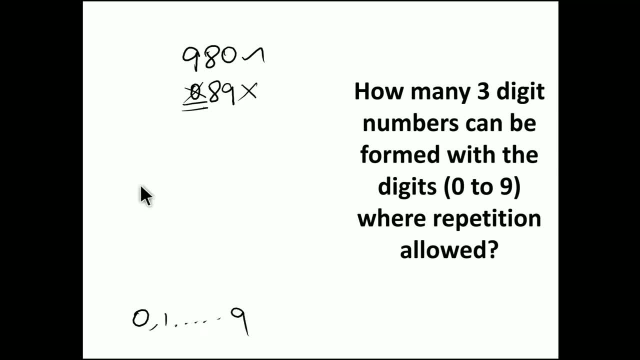 So you have number from 0 to 9. And you have to frame a 3 digit number. So first place cannot be 0, right, No? So first place can be filled in 9 ways by any one of these numbers, starting from 1 to 9.. 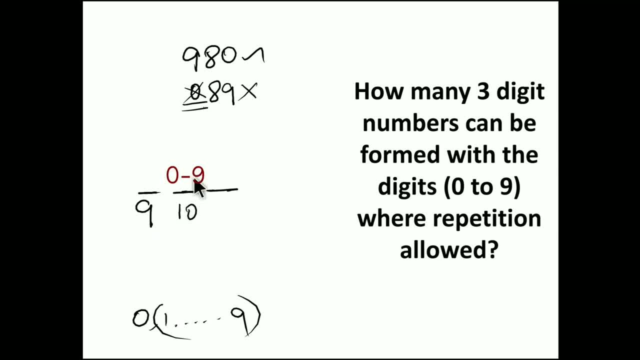 Now second place can be filled in 10 ways, because second place can be filled with 0, right? Similarly, third place can also be filled with 0. So any one of these 10 number will occupy the third place. So 9 into 10 into 10 is our answer. 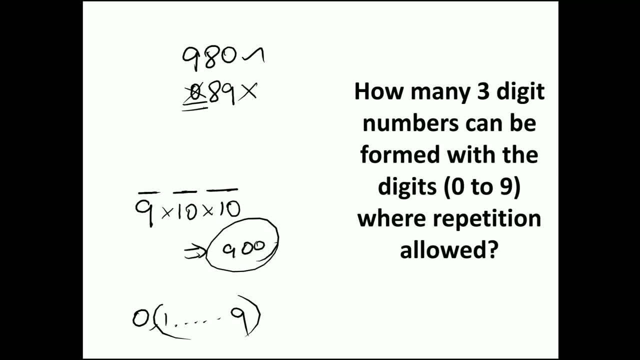 So, which is 900, 3 digit numbers can be formed with the digits 0 to 9, where repetition allowed. So here our concept is: first place cannot be filled with 0.. Hope you understood the concept right. Moving to last question of the video, 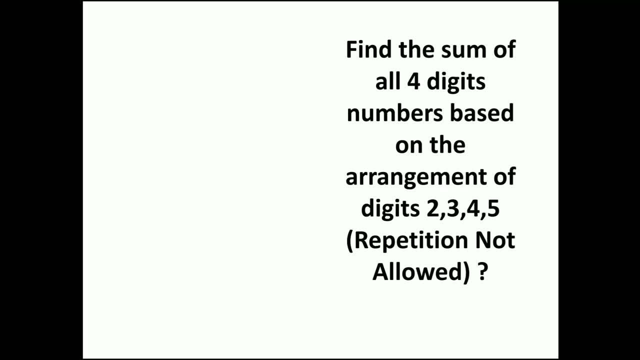 Find the sum of all 4 digit numbers based on the arrangement of the digits 2, 3, 4 and 5, where repetition not allowed. So if you observe this question closely, it seems to be little tricky, right? So let us move from most basic. 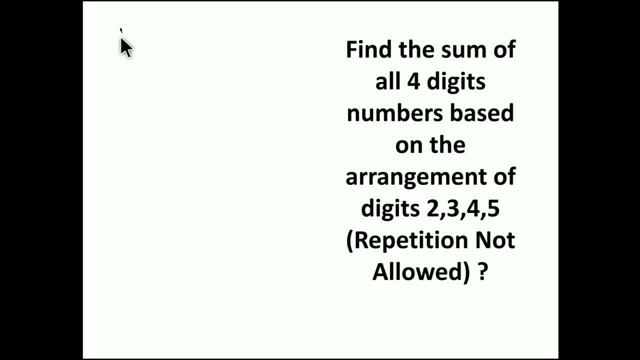 Assume, if you have a question like this, I give you 3 numbers: 1,, 2, 3.. And the question is: find the sum of all 3 digit numbers based on the arrangement of the given digits 1, 2 and 3, where repetition not allowed. 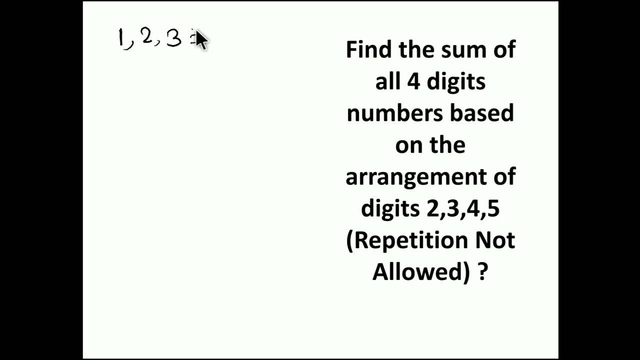 So how many arrangements are possible? So we can simply say you have to frame a 3 digit number right, 3 into 2, into 1, which is nothing but 3 factorial. So you totally get 6 arrangements from these numbers 1, 2 and 3.. 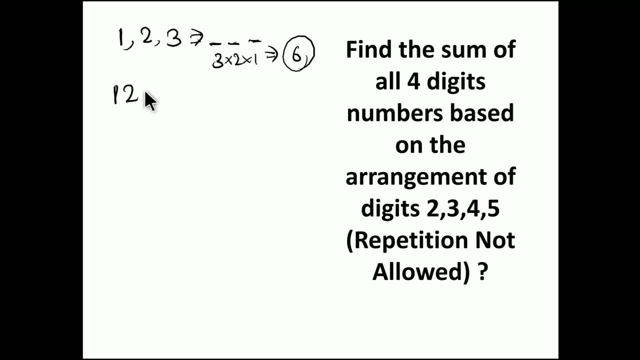 And if I want to write the arrangements: 1, 2, 3 is an arrangement. 2, 1, 3 is an arrangement. 3, 1, 2 is an arrangement. 1, 3, 2 is an arrangement. 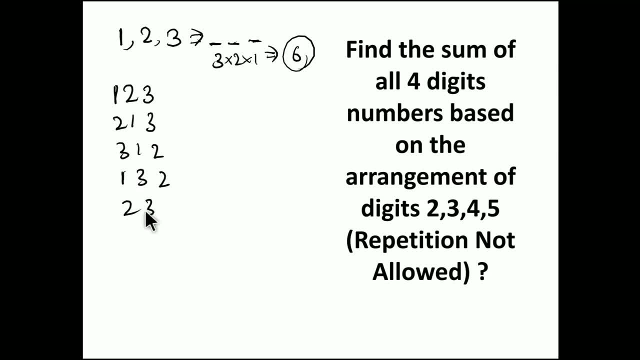 And 2, 3, 1 is an arrangement. 3, 2, 1 is an arrangement. You have to sum all these arrangements. So this is our question. Since these 3 numbers are simple, you can write it in this way: 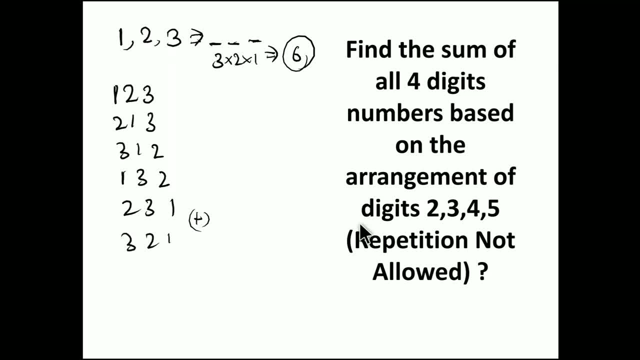 You can write using traditional way, But in this question you have 4 numbers, right? So 4 numbers in the sense you will totally get 24 arrangements. So 4 factorial is nothing but 24 arrangements, right? So you can't able to write all the arrangements. 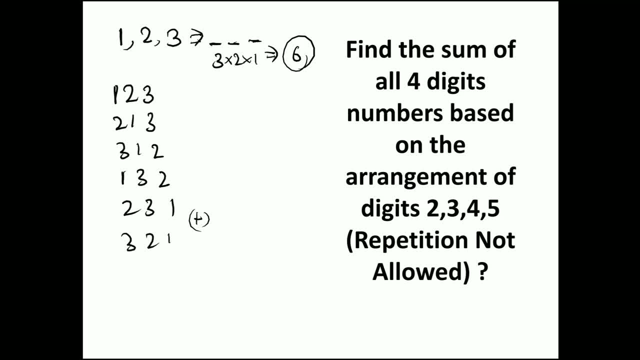 So if you sum it, it will consume 4.. It will consume lot of time where we can go with the short trick? Now you have to frame a 3 digit number right? So just try to keep a last digit constant. So here the last digit. if you keep last digit 3 constant, find total number of arrangements possible with the last digit ending with 3.. 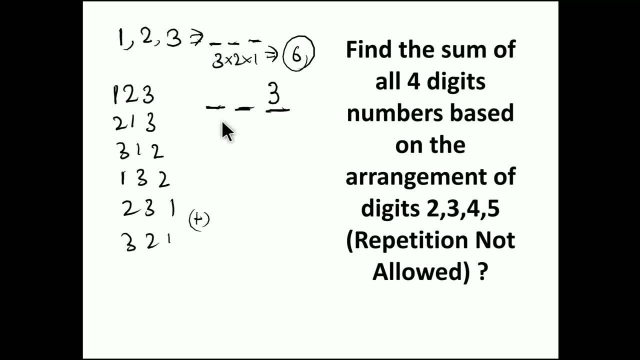 So if you keep 3 here, you are left with only 2 numbers. So first place can be filled in 2 ways and second place can be filled in 1 way. So 2 into 1, you get total 2 arrangements ending with 3, right. 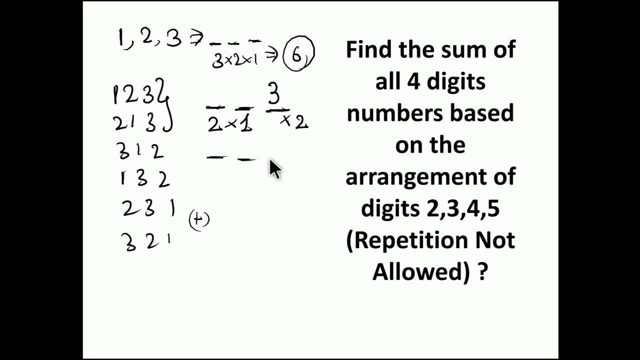 So you are getting 2 arrangements. Similarly, if you keep 2 at last, you will once again get 2 into 1, 2 arrangements possible. So it's nothing but 2, right? You are getting 2 arrangements: 3, 1, 2 and 1, 3, 2.. 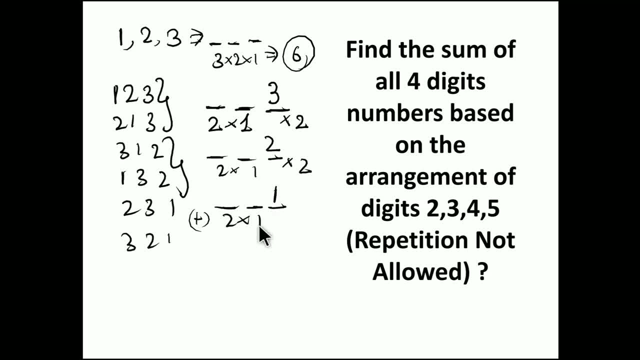 Similarly, if you keep the last digit, 1,, you will get 2 into 1.. So you will get 2 arrangements possible: 2, 3, 1 and 3, 2, 3, 2, 1, right. 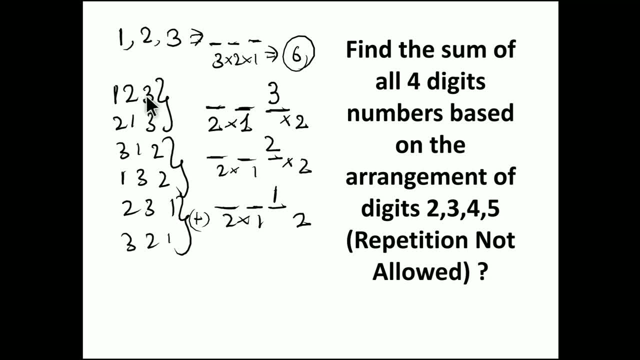 So you have to sum all the digits, right? So if you add 3 plus 3,, 6, 6 plus 2 plus 2, 4,, 10,, 10 plus 2. It's 12, right. 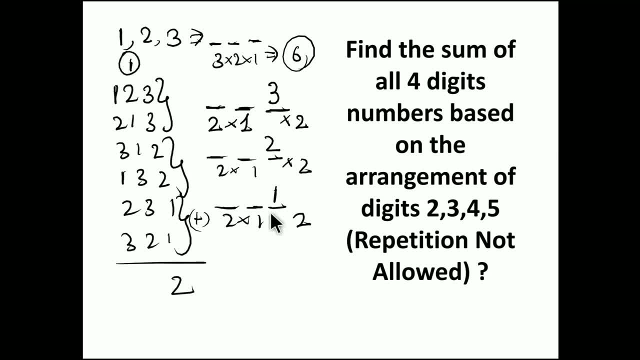 And you will get a carry 1.. So it's so simple here. Just multiply this 3 with 2, because you are getting 2 arrangements ending with 3, right? So 3 into 2, you get 6.. 2 into 2,, you get 4.. 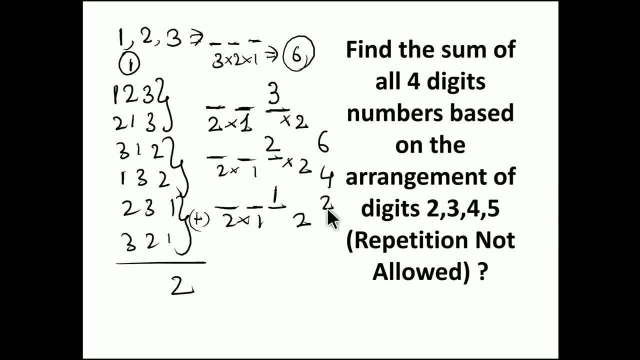 1 into 2, you get 4.. So 6 plus 4, 10.. 10 plus 2, 12.. So here the last digit is 2 and you have a carry 1.. Similarly, if you add all these 10s place, you will get once again 12.. 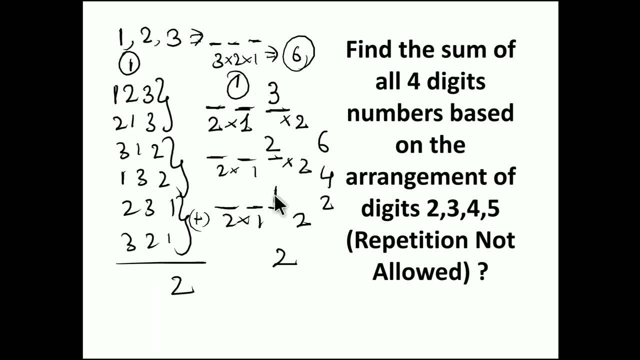 So if the last digit here is 12.. If you sum all these digits, if you are getting 12, once again, you will get 12 when you sum all the 10s place. So 12 plus 1, you get 13.. 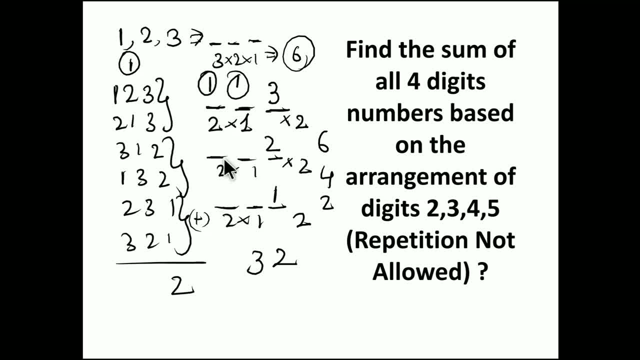 So once again you will get a carry 1.. So if you add all the 100s place, you will get a 12.. So 12 plus 1, you get 13.. So 1, 3, 3, 2 is the sum of all 3 digit numbers based on the arrangement of the given digits, 1, 2 and 3.. 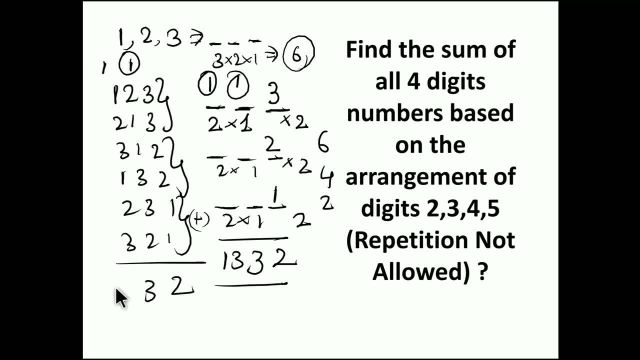 So, once again, if you add all this, you will get a 3 here and 1 here and a 13.. However, the answer remains same. I hope you understood the concept right. By applying the same concept, we are going to solve the problem here. 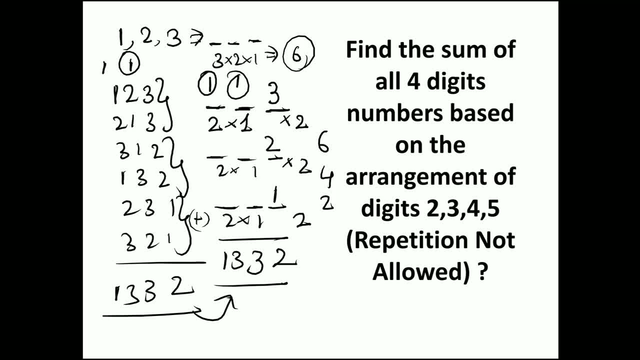 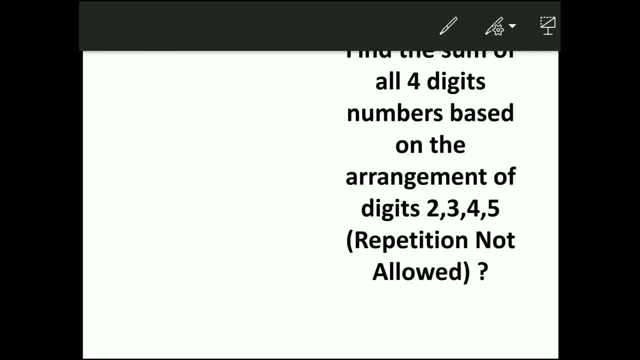 Find the sum of all 4 digit numbers based on the arrangement of digits 2,, 3,, 4 and 5, where repetition is not allowed. Now we know, from the digits 2,, 3,, 4 and 5, we totally get 24 arrangements. 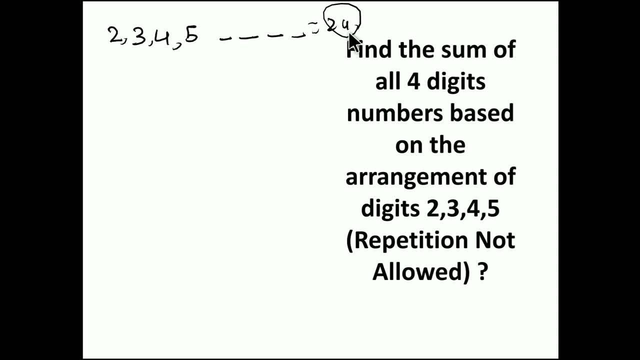 4 x 3 x 2 x 1, we totally get 24 arrangements. Now keep the last digit as 5,, which is the constant. Now, first place can be filled in 3 ways. So if you keep 5 constant, you are left with 3 numbers. 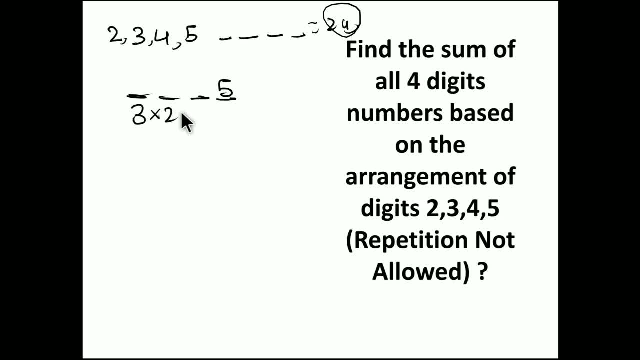 So first place can be filled in 3 ways, second place in 2 ways and third place in 1 way. So 3 x 2 x 1, you totally get 6 arrangements ending with 5.. Similarly, if you keep last digit, 4, you will get 6 arrangements ending with 4.. 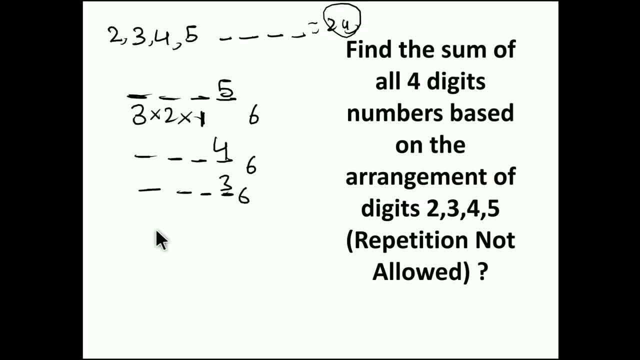 If you keep the last digit, 3,, you will get 6 arrangements ending with 3.. For 2 also, you will get a 6 arrangement ending with 2.. So 5 x 3 x 1 is the same 6. see if you get the last digit 5 and 6 arrangement. if you add 5 for 6 times, you will get 30 right. 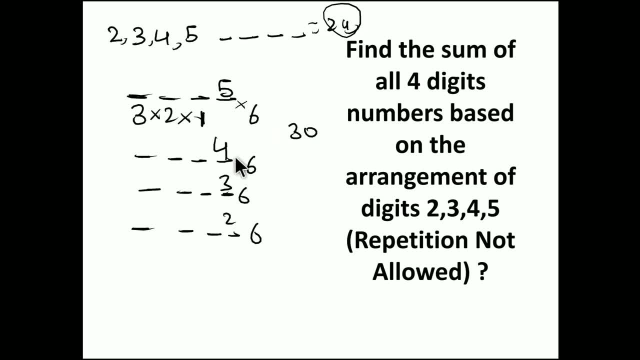 so simply multiply 5 with 6, you get 30. 4 into 6, you get 24. 3 into 6, you get 18. 2 into 6, you get 12. when you add all these numbers, you will get 84 right. that means the last. 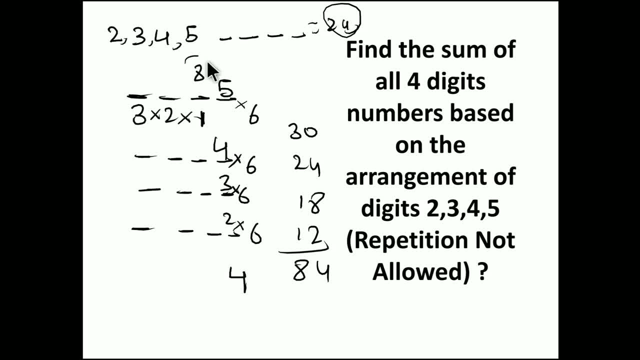 digit will be 4 and the carry is 8, and which will move to 10 space. once again. if you add all the 10 space, you will get 84, 84 plus 8, you get 92 and carry is 9, and which will 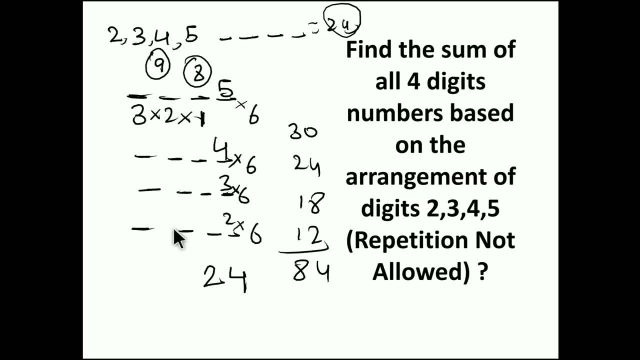 sit in 100 space. once again, if you add all the 100 space, you will get 84. only 84 plus 9, you get 93 and the 9 will sit in 1000 space. if you add all the 1000 space, once again, you 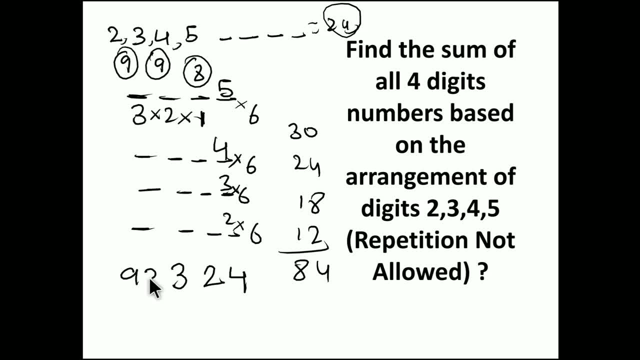 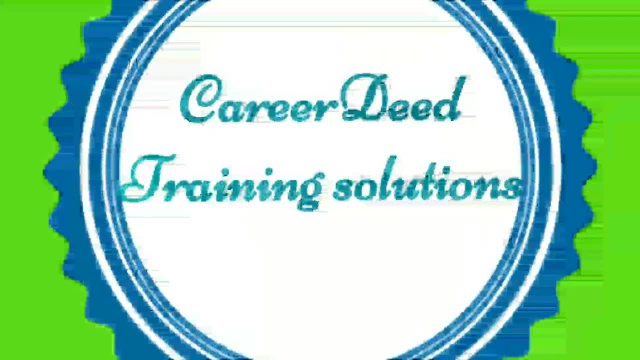 will get 84, 84 plus 9, you get 93. so 9, 3, 3 to 4 is the answer for the particular question. now the next choix question is going to be asked in the table. wright, well, the first question is not answered, so we have a three by three solution. we need to discuss our solution.